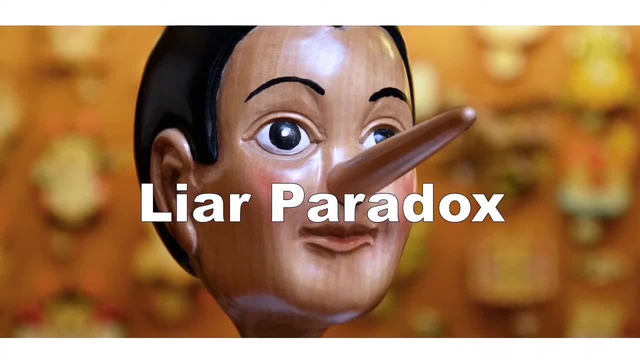 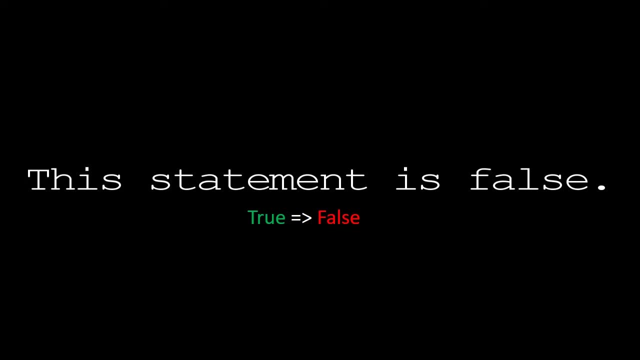 Hello there. You have probably heard of the liar paradox which asks whether the statement is true or false. Of course, the paradox here is that if you say it's true, then the statement itself says it's false, and if you say it's false, then the statement correctly says it's. 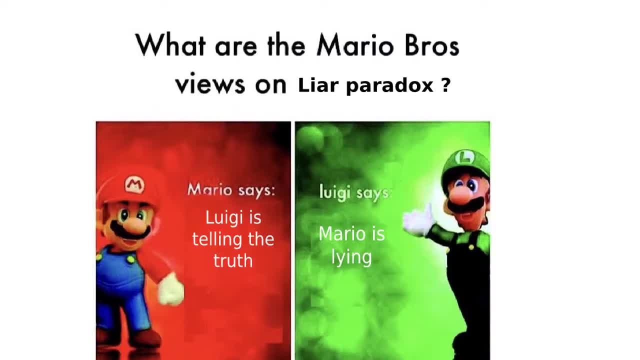 false making it true. This sort of self-referencing, paradoxical statements can always be constructed quite easily in English. We are, however, not particularly concerned about these, because we don't expect sentences in English to be either true or false. It, however, is not. 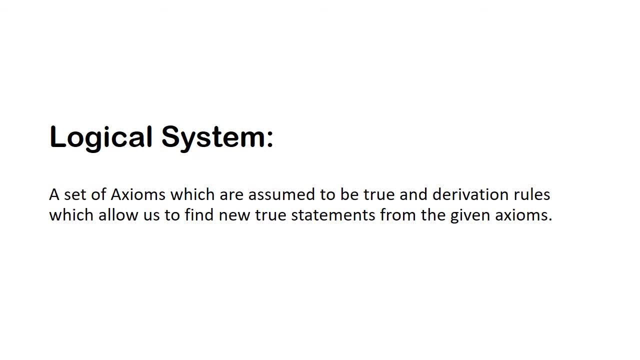 the case in logic. Now, in logic, a logical system is a set of axioms or facts which we have assumed to be true and a set of derivation rules which allow us to find new true statements from the given axioms Every statement in a logical system does indeed need to have. 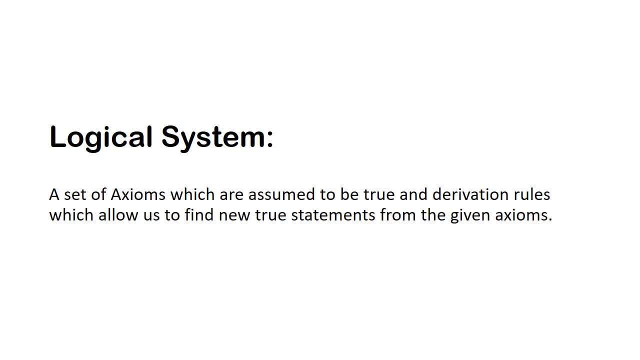 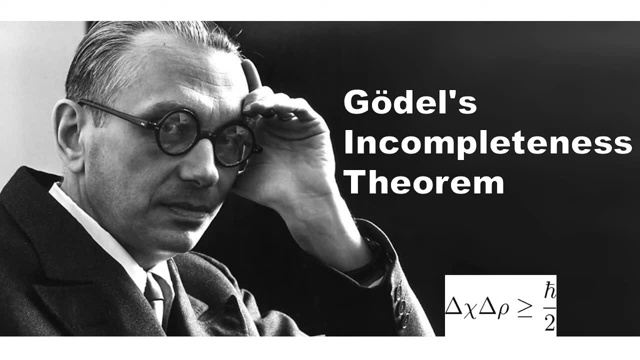 a truth value. Now, if we could find a paradox, as before inside the logical system, we would reach Godel's incompleteness theorem, one of the most ground-breaking theorems from the 20th century, On par with Heisenberg's uncertainty principle or Einstein's theory of relativity, in terms 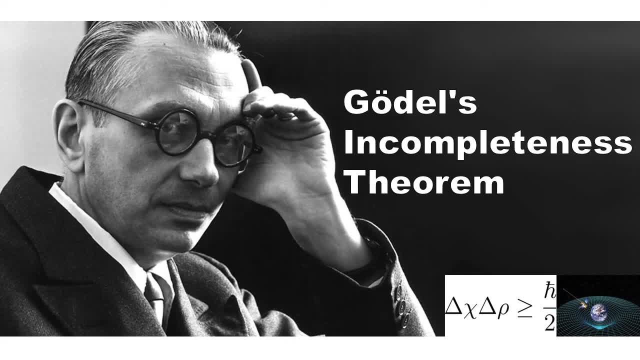 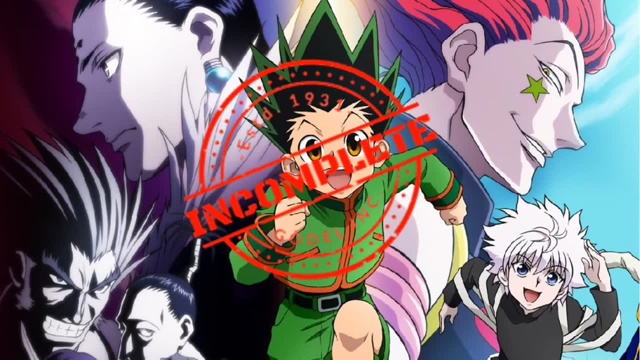 of ground-breakingness. it says, in its most simplified and click-baity version, that math is incomplete. Now you may wonder: why are we worried about that? There are several incomplete things in life, and to answer that we must first talk about what it means to be complete. 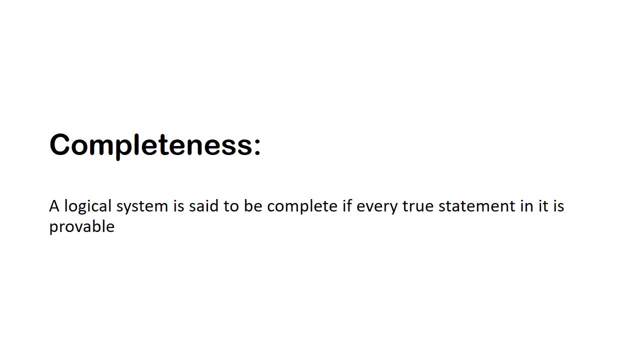 in logic. A logical system is said to be complete if every true statement in it can be proved. So what the theorem says is: there are true statements in mathematics that cannot be proved. This is unsettling because since the time of the ancient Greeks, mathematicians 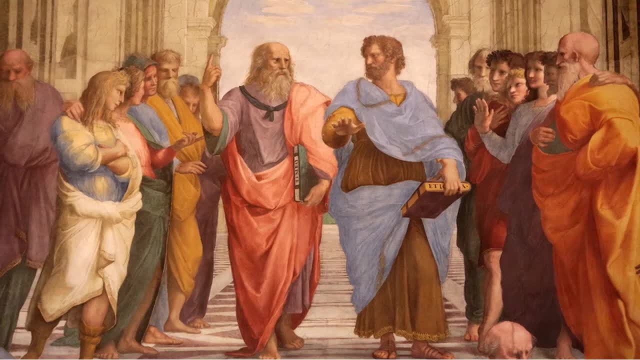 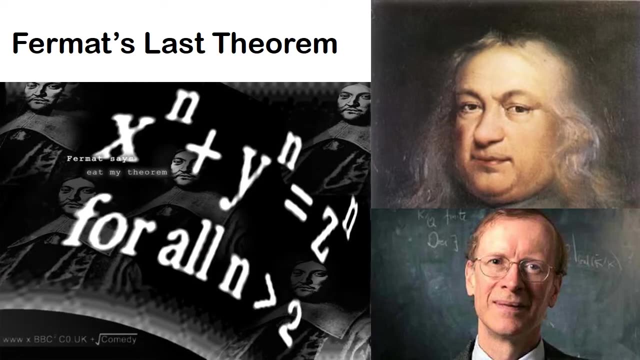 have intuitively had the idea that any true statement must be provable. Of course, that proof might be difficult, or perhaps very, very difficult, but provable nevertheless. However, Godel's incompleteness theorem says that the problems that you might have been 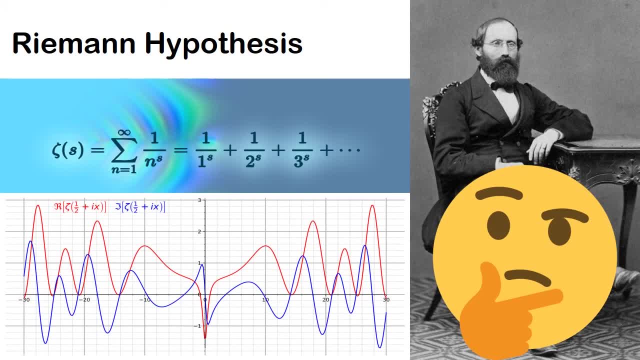 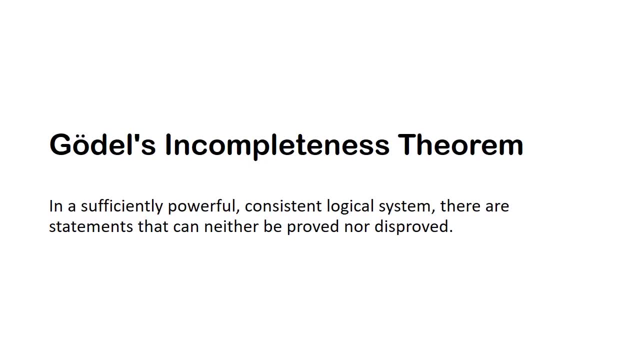 working on for years might not actually be solvable at all, despite being true. Now, coming back to the theorem itself, let's look at a less click-baity version of the definition In a sufficiently powerful, consistent and easy-to-understand mathematical system, the 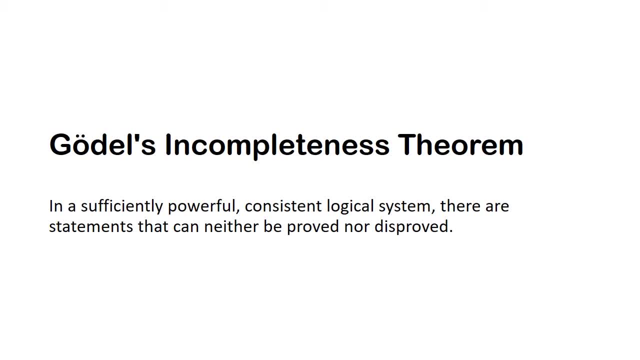 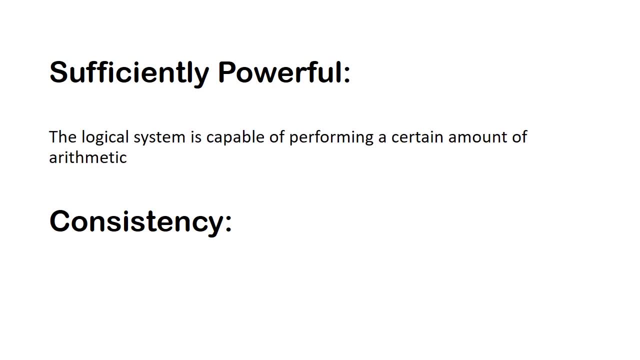 statements can neither be proved nor disproved. To start off, by sufficiently powerful we mean the logical system can carry out a certain amount of arithmetical operations, and by consistent we mean it is impossible to prove both a statement and its opposite in the logical. 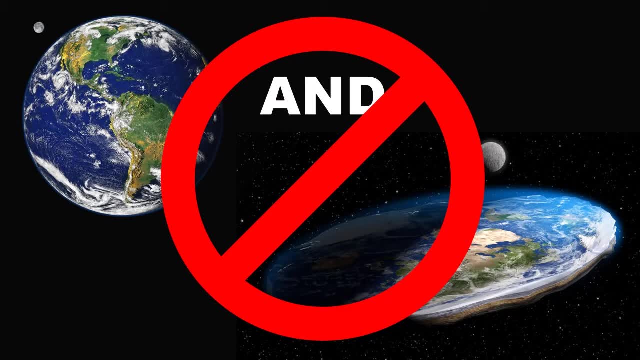 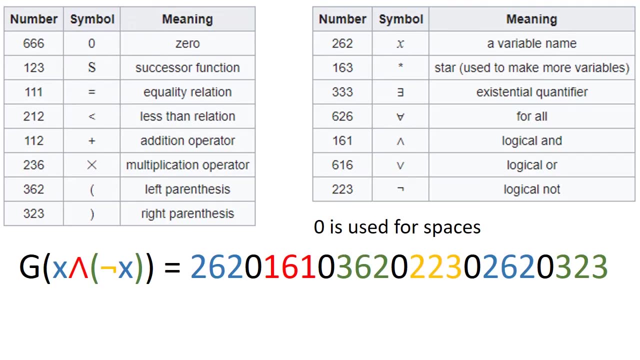 system. For example, we can't prove both earth is round and earth is flat using a consistent logical system. To start off proving this, the first step is to encode every logical formula f as the natural number. g, which Godel referred to as Godel numbering The. 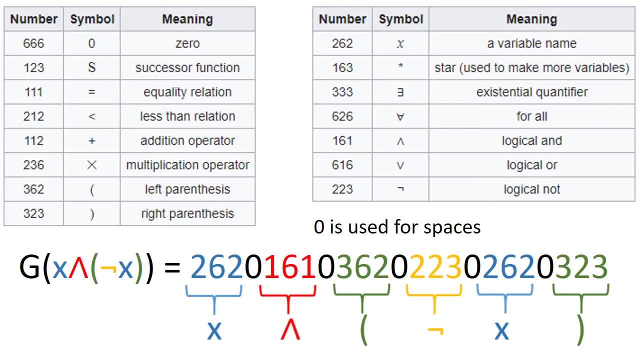 idea is to assign the natural number to each symbol and then build up statements by putting together the natural numbers associated with the symbols of that statement. This is quite similar to binary encoding that is used by computers everywhere. Now, with the natural number associated with every formula, we can define the properties. 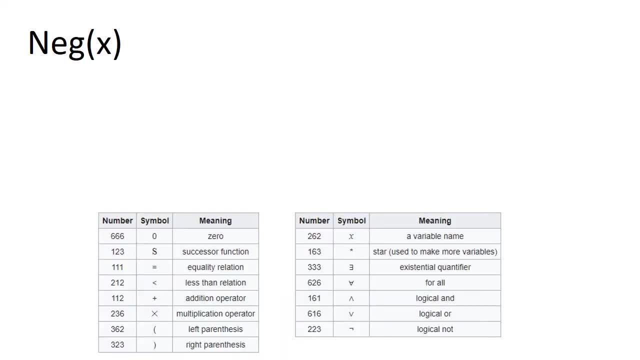 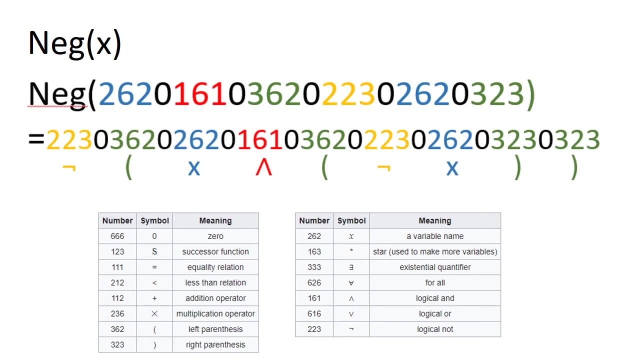 of logical formulas using numbers. For example, we can have a function- negation of x on numbers- which sends x, which is a natural number, to the Godel number of the negation of the logical formula associated with x. Another thing to note is we can determine using computer: 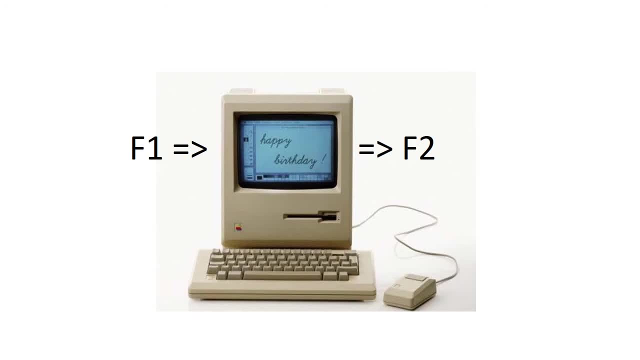 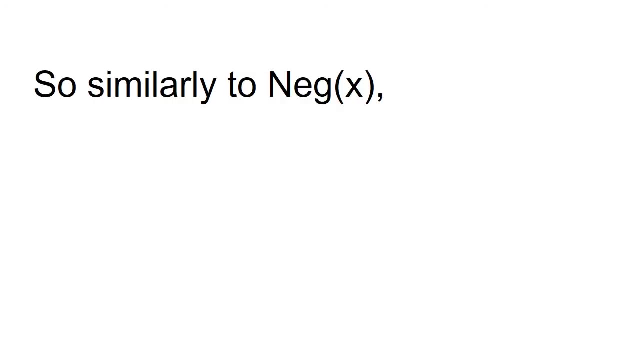 programs, whether for two formulas, f and f. f is a proof of f, since proofs and logic are basically just logical formulas themselves. Using this fact, we can have a function proof of x which returns true if the formula associated with the number x proves the formula associated with the number y, given they are valid formulas. 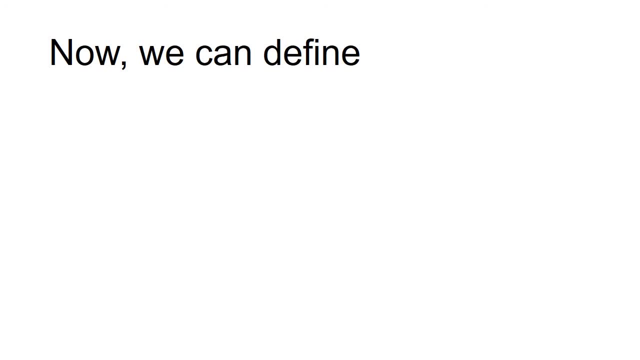 Now we can define provability of the logical formulas in the terms of natural numbers, as a formula x is provable if there exists a logical formula y such that y proves x, So provable of x can be defined as there exists y such that proof of y of x. 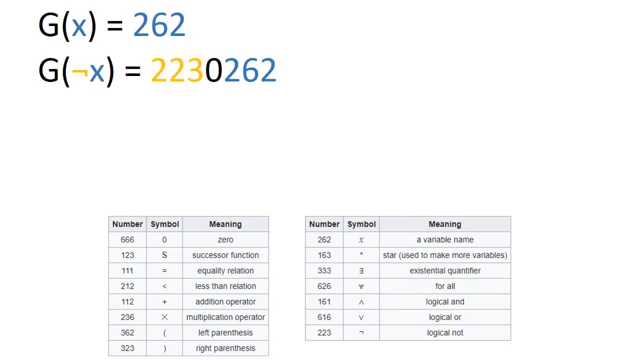 Now remember that each logical formula is tied to a natural number by the Godel numbering. so we can arrange all formulas which take one free variable as input in ascending order, in the order of its Godel number. This way we create a list of logical formulas with. 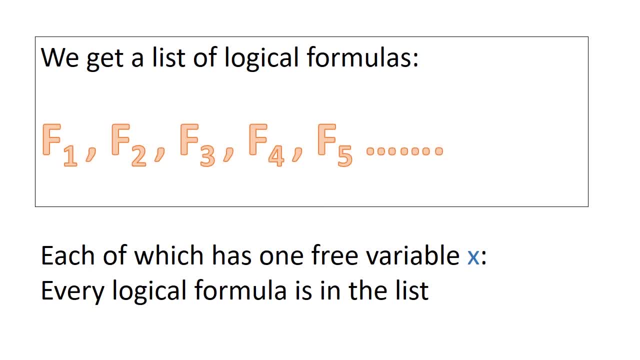 one free variable, such that every logical formula with one free variable is in that list. Again, they are functions over natural numbers, so not only are they indexed by natural numbers, they also take natural numbers as arguments. Now consider the formula D, where